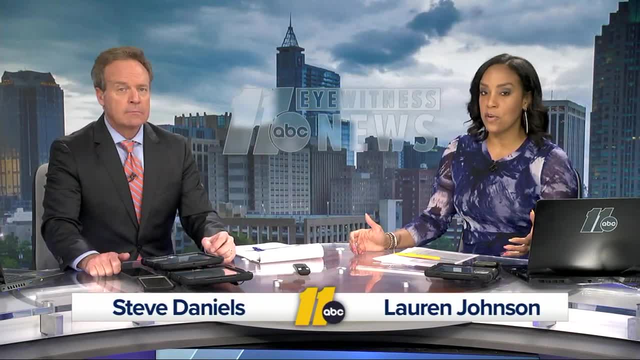 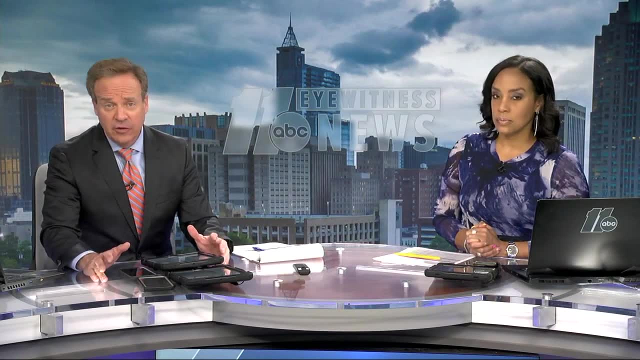 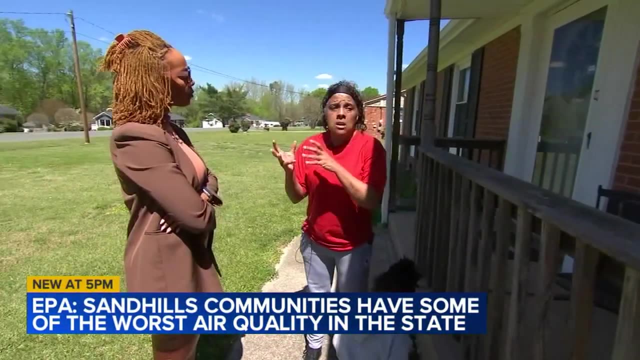 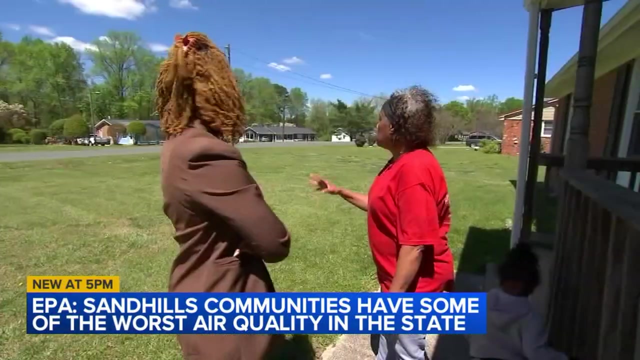 New at 5,: what's in the air where you live? Eyewitness News uncovering data from the EPA that shows communities in the Sandhills have some of the worst air quality in our state. People living there believe they have health conditions. to prove it, Racing culture reporter Akilah Davis has the story now from Lee County. The air is so dry you'd expect to see open windows on this breezy spring day, But at Terry Petty's Sanford North Carolina home that's not an option. Most of us keep our windows closed 95% of the time. The 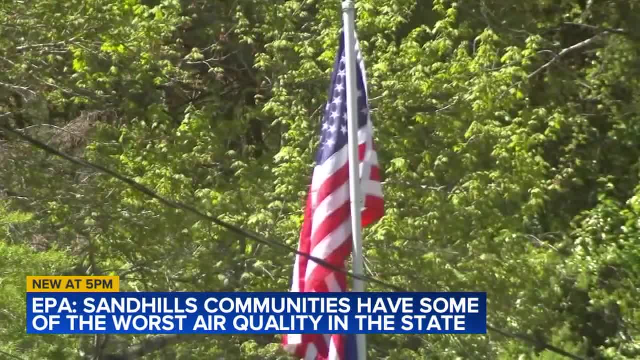 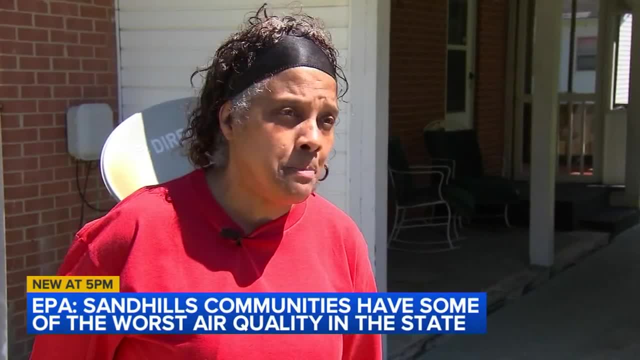 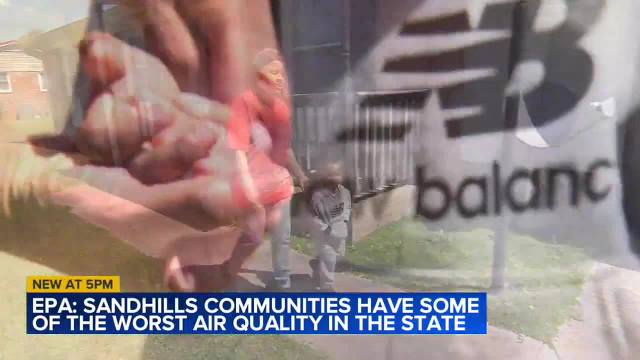 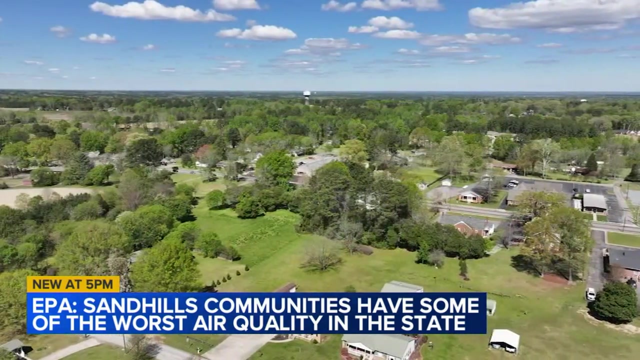 63-year-old, is proud to live in Kendall Acres, a close-knit community and one her father fell in love with more than 30 years ago. One thing that stood out to him: that the yard was big- Big enough for her two-year-old nephew, Kyrie, to play in. Come on Fats. She's careful not to have him outdoors much. Sometimes his skin will get real dry and I think it comes from the air. Minor concerns compared to what she and her neighbors are experiencing. It does something to my throat. A lot of people have asthma. 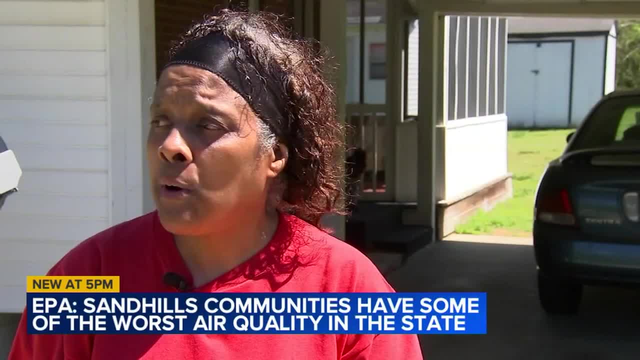 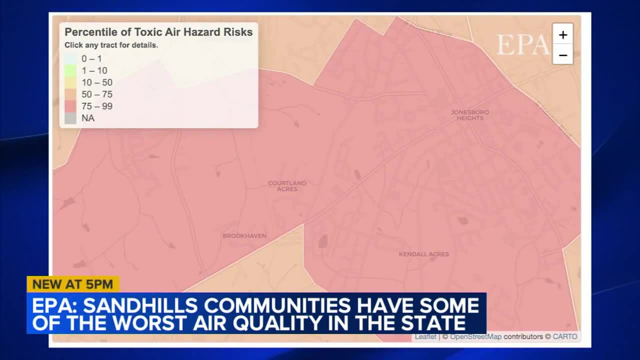 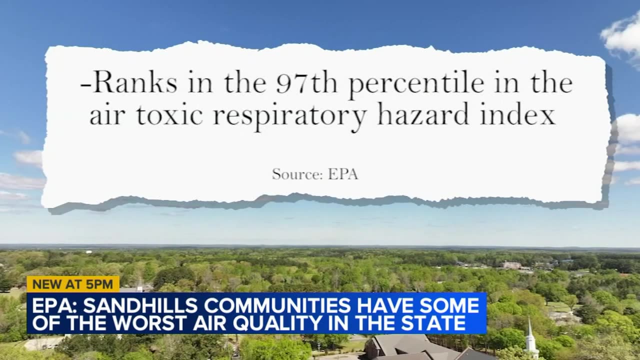 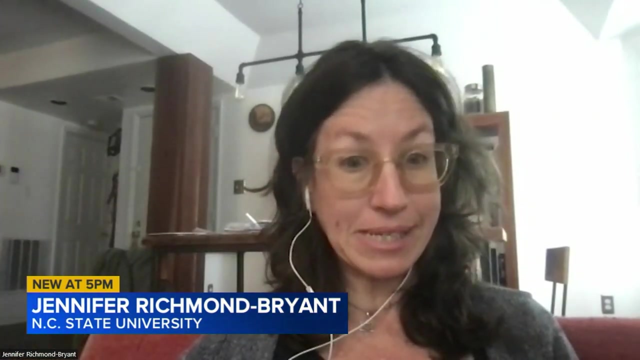 and I know a lot of people on my street have COPD but it comes from smoking. but some folks don't even smoke. Data from the EPA shows these communities in Sanford have some of the worst air quality in the state, ranking in the 97th percentile in the Air Toxics Respiratory Hazard Index. It means that a lot of pollutants are being emitted at lower levels but because there are a lot of them, they're contributing to the air quality of the state. 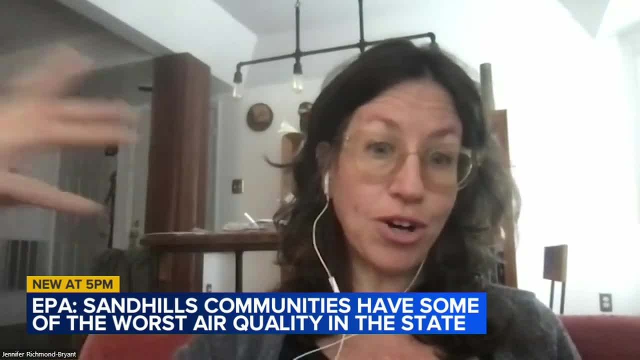 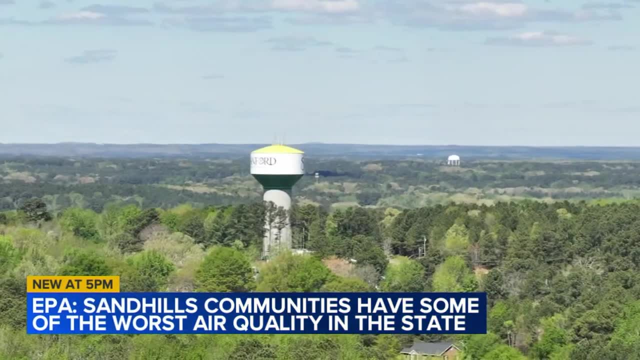 They're contributing to the air quality of the state. унitron roar- A lot of people said they don't even smoke and most of the stations are repaying, distributing the �aa Demands, because they're also contributing to the overall air pollution load in the area. Jennifer Richmond Bryant is a NC State professor working in the college of Natural Resources. She's 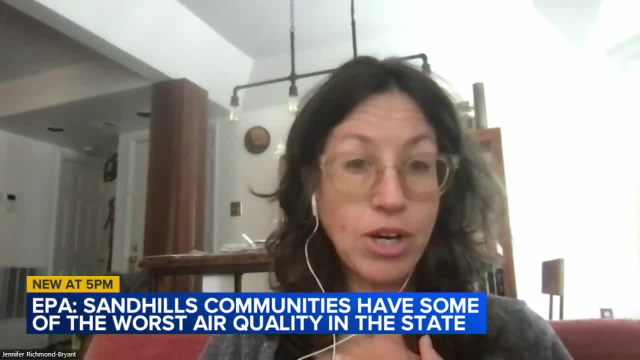 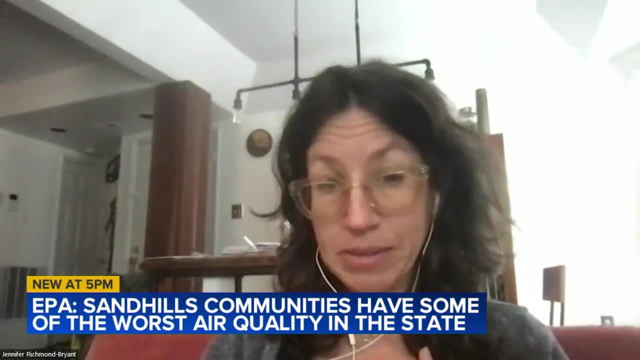 She's worked for the EPA for over a decade. if I myself was having something like shortness of breath or, um, trouble breathing, or asthma for that matter, That would be Other drugs causes for concerns down. the data also shows people living here are mostly from communities of color and here